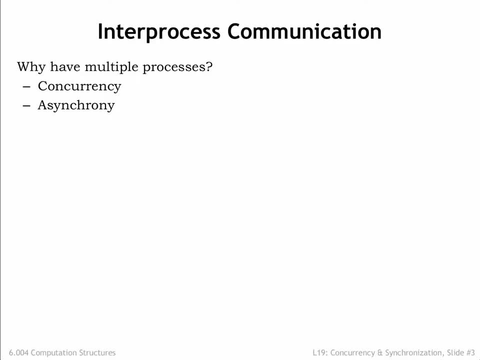 to organize the processing of user events separately from the back-end processing Processes are an effective way to encapsulate the state in computation for what are logically independent components of an application which communicate with one another when they need to share information. These sorts of applications are often data- or event-driven, in other words, the process. 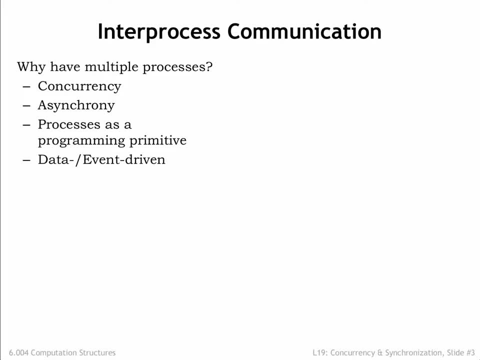 processing required is determined by the data to be processed or the arrival of external events. How should the processes communicate with each other? If the processes are running out of the same physical memory, it would be easy to arrange to share memory data by mapping the same physical page into the contexts for both processes. 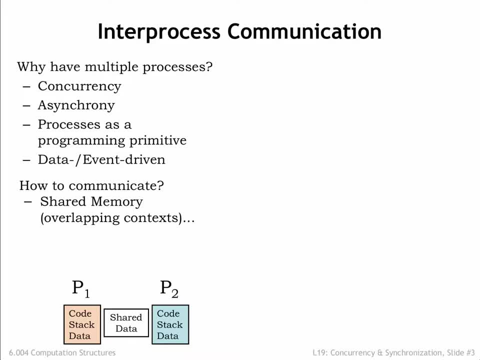 Any data written to that page by one process will be able to be read by the other process. To make it easier to coordinate the processes, we can use the same memory data To coordinate the processes communicating via shared memory. we'll see it's convenient. 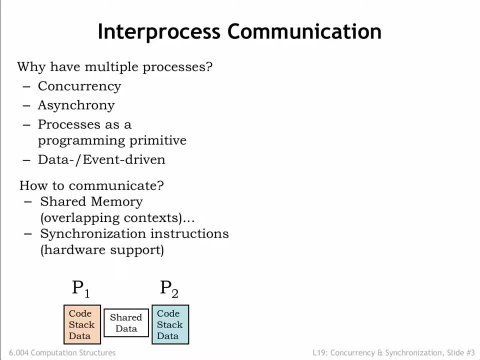 to provide synchronization primitives. Some ISAs include instructions that make it easy to do the required synchronization. Another approach is to add OS supervisor calls to pass messages from one process to another. Message passing involves more overhead than shared memory but makes the application programming. 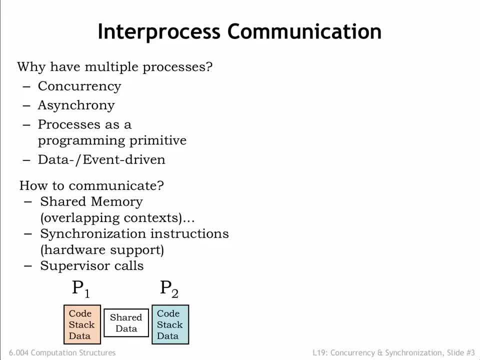 environment, independent of whether the communicating processes are running on the same network. If the processes communicate via shared memory, we'll see it's convenient to provide synchronization primitives. In this lecture we'll use the classic producer-consumer problem as our example of concurrent processes. 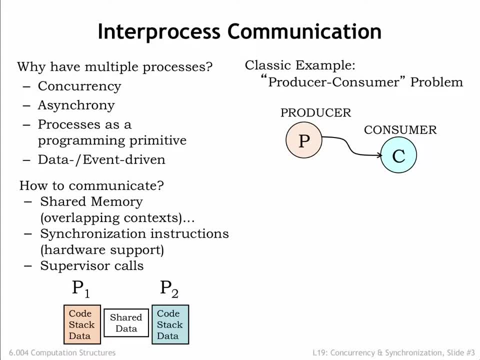 that need to communicate and synchronize. There are two processes: a producer and a consumer. The producer is running in a loop which performs some computation to generate information. The consumer is also running in a loop which waits for the next character to arrive from the producer, then performs some computation. 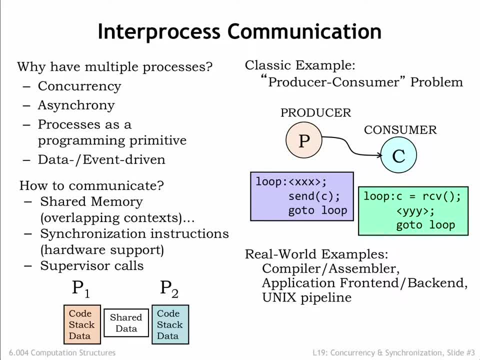 The information passing between the producer and consumer could obviously be much more complicated than a single character. For example, a compiler might produce a sequence of assembly language statements that are passed to the assembler to be converted into the appropriate binary representation. The user interface frontend for a video game might pass a sequence of player actions to. 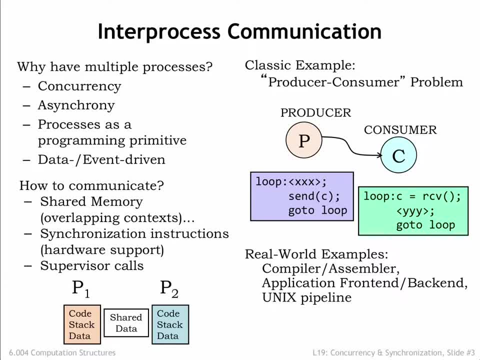 the simulation and rendering backend, And so it's simple. In fact, the notion of hooking multiple processes together in a processing pipeline is so useful that the UNIX and Linux operating systems provide a pipe primitive in the operating system that connects the output channel of the upstream process to the input channel. 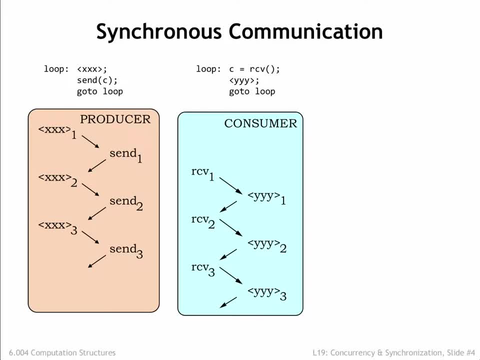 of the downstream process. Let's look at a timing diagram for the actions of our simple producer-consumer example. We'll use the arrows to indicate when one action happens before another Inside a single process. the order of execution implies a particular ordering and time. 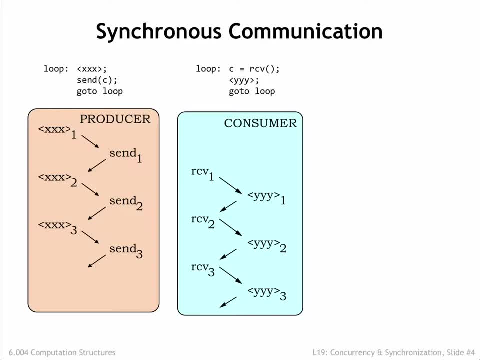 The first execution of XXX is followed by the sending of the first character. Then there's the second execution of XXX, followed by the sending of the second character, and so on. In later examples we'll omit the timing arrows between successive statements in the same. 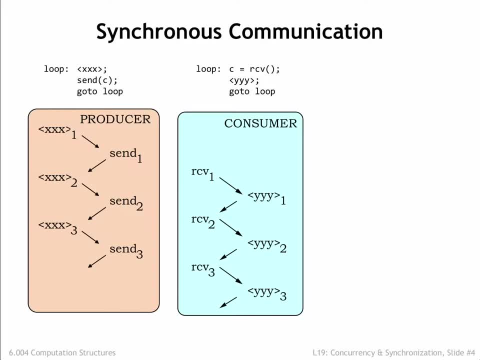 program. We see a similar order of execution in the consumer: The first character is received, Then the computation YYY is performed for the first time, etc. Inside of each process the processes program counter is determining the order in which computations are performed. 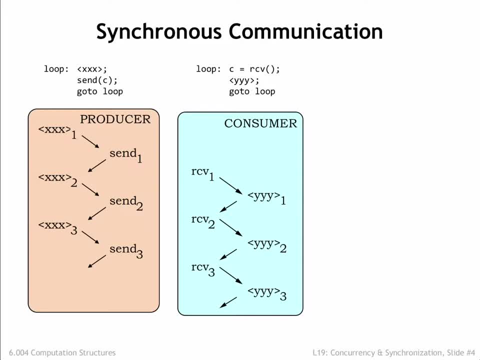 So far, so good. each process is running as expected. However, for the producer-consumer system to function correctly as a whole, we'll need to introduce some additional constraints on the order of execution. These are called precedence constraints, and we'll use the stylized less-than sign to end. 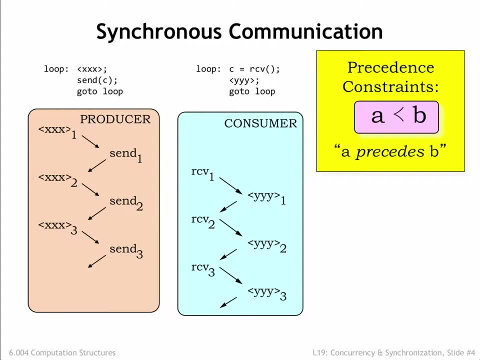 the operation. These constraints indicate that a computation A must precede, ie come before, computation B. In the producer-consumer system we can't consume data before it's been produced. a constraint we can formalize as requiring that the ith send operation has to precede the 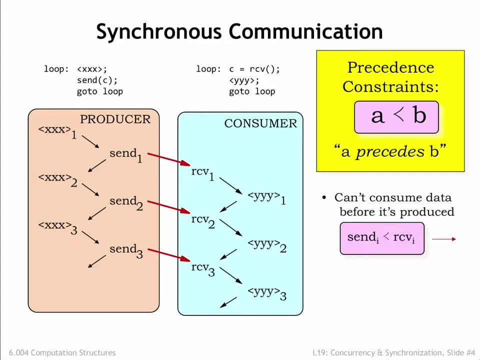 ith receive operation. This timing constraint is shown as the solid red arrow in the timing diagram. Assuming we're using, say, a shared memory location to hold the character being transmitted from the producer to the consumer, we need to ensure that the producer doesn't. 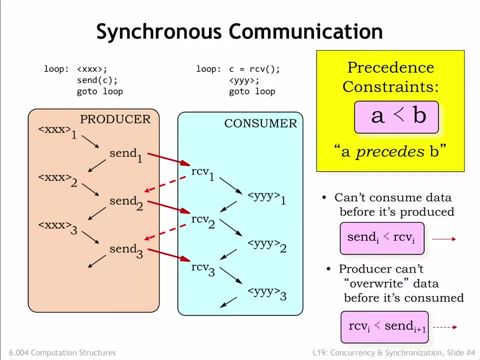 overwrite the previous character before it's been read by the consumer. In other words, we require the ith receive to precede the ith-plus-first send. These timing constraints are shown as the dotted red arrows in the timing diagram. Together, these precedence constraints mean that the producer and consumer are tightly. 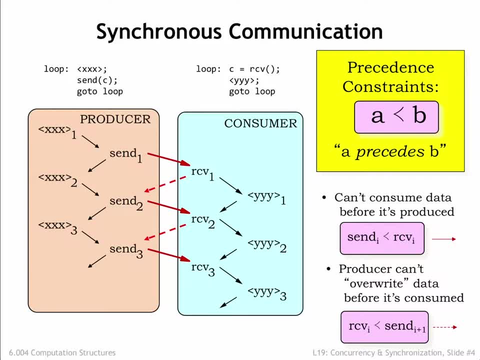 coupled in the sense that a character has to be read by the consumer before it's been sent by the next character, which might be less than optimal if the xxx and yyy computations take a variable amount of time. So let's see how we can relax the constraints to allow for more independence between the 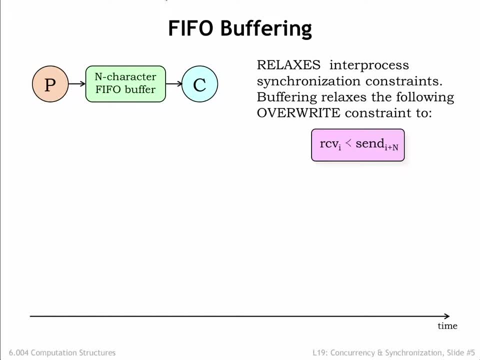 producer and consumer. We can relax the execution constraints on the producer and consumer by having them communicate via an n-character first-in, first-out buffer. That's right. As the producer produces characters, it inserts them into the buffer. The consumer reads characters from the buffer in the same order as they were produced. 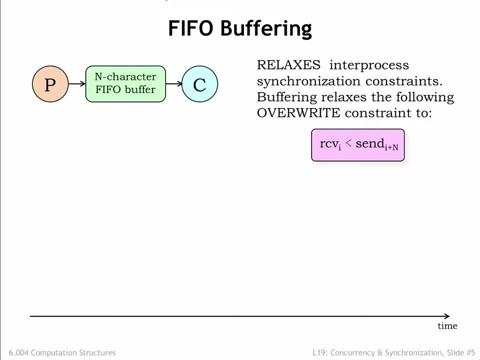 The buffer can hold between 0 and n characters. If the buffer holds 0 characters, it's empty. If it holds n characters, it's full. The producer should wait if the buffer is full. The consumer should wait if the buffer is empty. 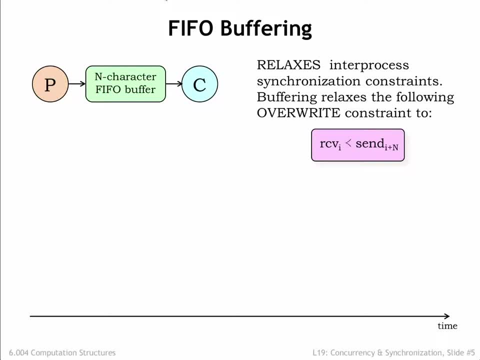 Using the n-character FIFO buffer relaxes our second overwrite constraint to the return requirement that the i-th received must happen before the i plus n-th send. In other words, the producer can get up to n characters ahead of the consumer. FIFO buffers are implemented as an n-element character array with two indices. 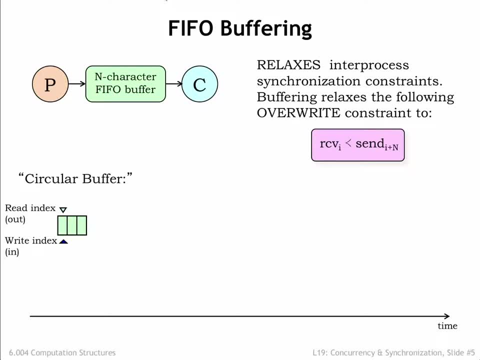 The read index indicates the next character to be read. the write index indicates the next character to be written. We'll also need a counter to keep track of the number of characters held by the buffer, but that's been omitted from this diagram. The indices are incremented modulo n, in other words, the next element to be accessed after. 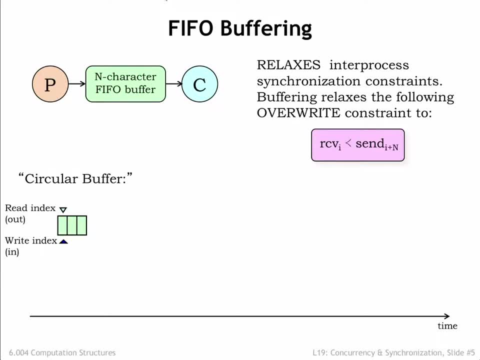 the n-1st element is the 0th element, hence the name: circular buffer. Here's how it works. The producer runs using the write index to add the first character to the buffer. The producer can produce additional characters but must wait once the buffer is full. 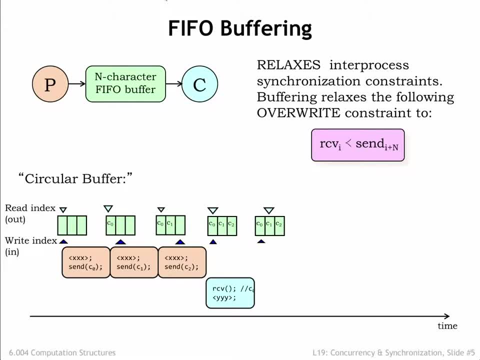 The consumer can receive a character any time the buffer is not empty, Using the read index to keep track of the next character to be read. Execution of the producer and consumer can proceed in any order so long as the producer doesn't write into a full buffer and the consumer doesn't read from an empty buffer.